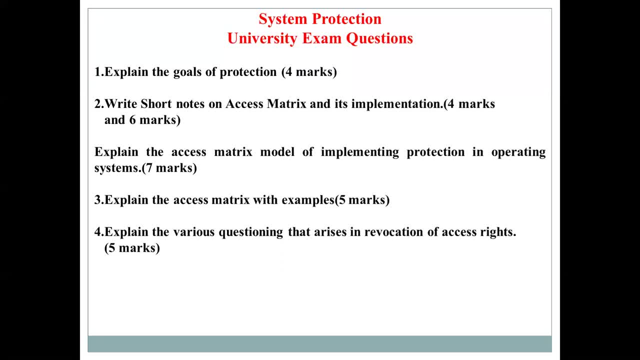 So, hello everyone. In this series of lectures, let's learn about the concept of system protection in operating systems. So, before learning about the concept of system protection, I've just presented you a screenshot of the different university exam questions which has been asked. 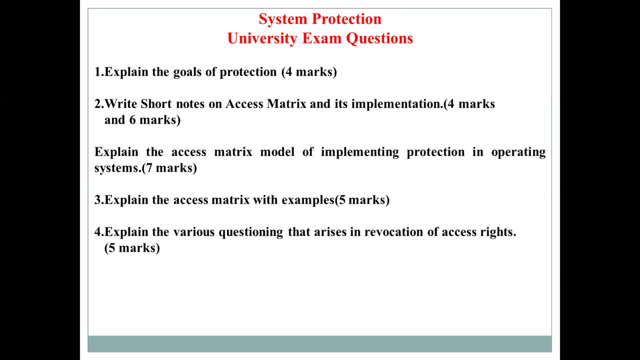 in this topic of system protection. So the first topic which I'll be taking in this series of lectures will be about goals of protection- Now that has been asked in many university exams for four months. And then another frequently asked question is about the concept of access. 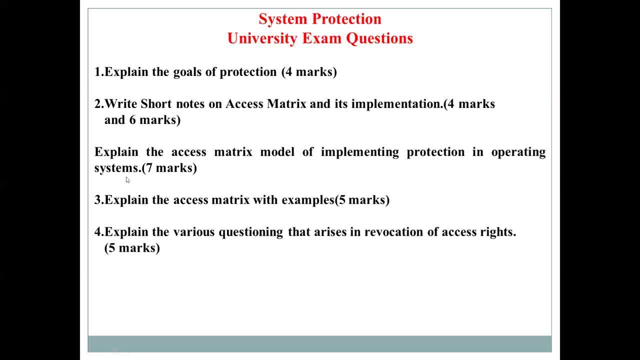 matrix, And the next frequently asked question is about the implementation of the access matrix model. One thing which you have to remember here is that the concept of access matrix is different from the implementation of access matrix. So right, short notes on access matrix deals with what is access matrix and how it helps to achieve the concept of 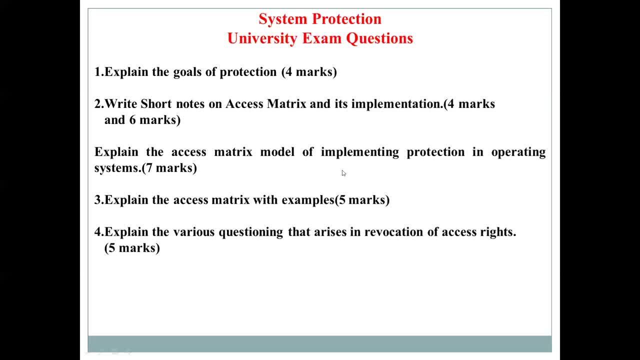 system protection. But then implementation of access matrix actually deals with how you can implement it. what data structures can be used for implementing that concept. So try to understand the question in depth when it is asked in the examination. Try to understand what they are trying to. 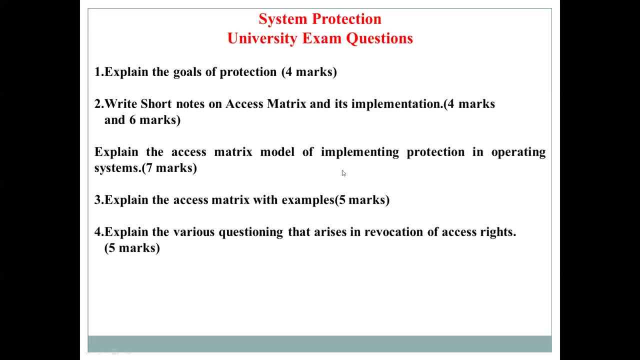 ask you to write whether you are asked to write about access matrix or about the implementation of access matrix, And then understand it and then start writing the answer, And then that is being asked for four to seven marks, And then done So. the next question which is asked in this concept of system protection is about 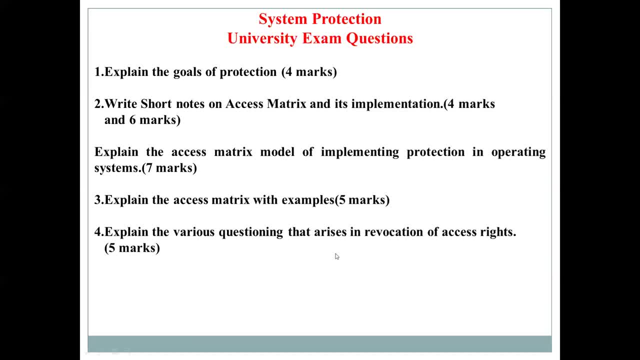 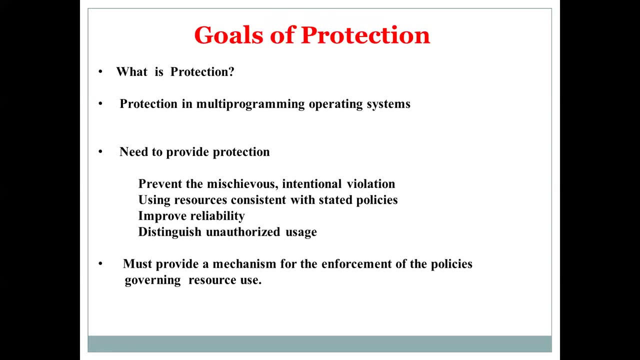 the revocation of access rights, which will be the last topic in this series of lectures. So now in today's lecture let us see about the concept of goals of protection and about the principles of protection. So first topic is about the Goals of Protection. So first of all, 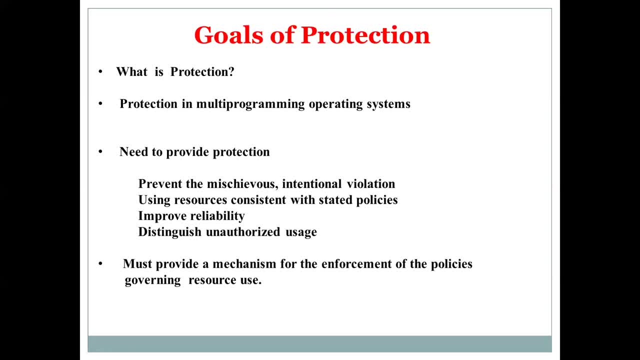 before knowing about the goals of protection, I should know what is the meaning of protection. So the first going to be the goals of protection. first of all, with respect to preparation, I should know what is the meaning of protection by the sorry. 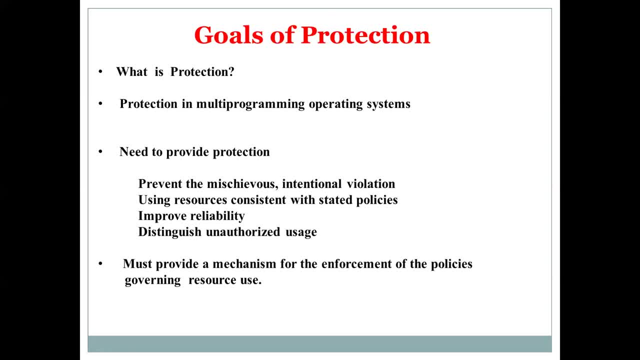 of protection and why I need protection. so protection is: just imagine a typical multi programming environment. in a typical multi programming environment, multiple programs are going to be there in the memory at the same time, so that means the OS has to prevent one process from accessing the address space of. 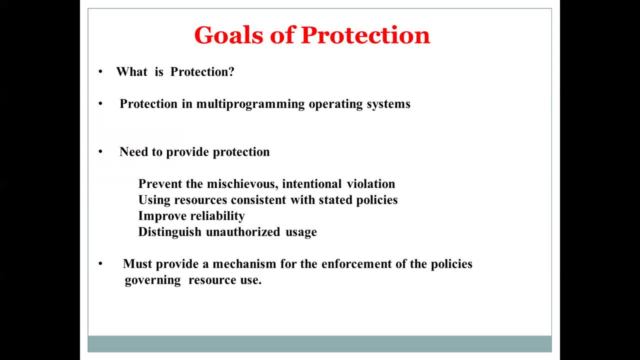 another process- and that is one of the main goals. one process when multiple processes are going to be there in memory at the same time. one program or the process should not be able to access that the space of the OS or the address bass of the of other process. that is one of the goods. 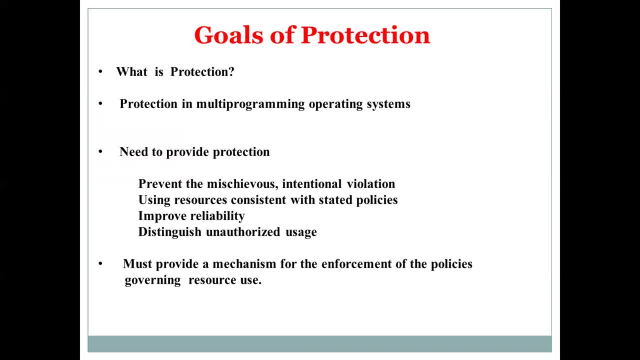 another goal is whenever, whenever any process is accessing the file or the memory segment or the CPU or any other system resource, only authorized, proper, authorized processes should be able to gain access. okay, unauthorized process should not be able to access to the CPU or the input. angry lazers or 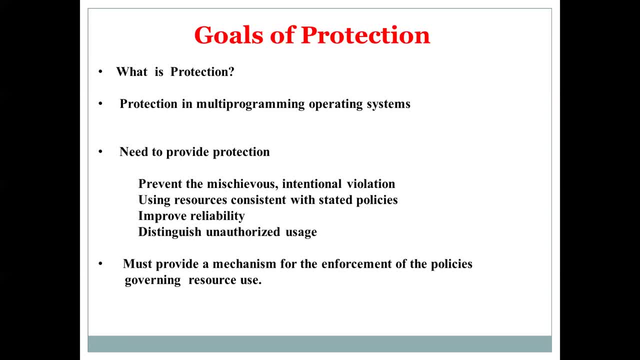 to any or to any resource of the computer system. so that is the main goal of protection. okay, so protection is dealing about. protection is about ensuring that all these things are in place. so if you if for a formal definition, we can say the protection is nothing, but it's the mechanism. 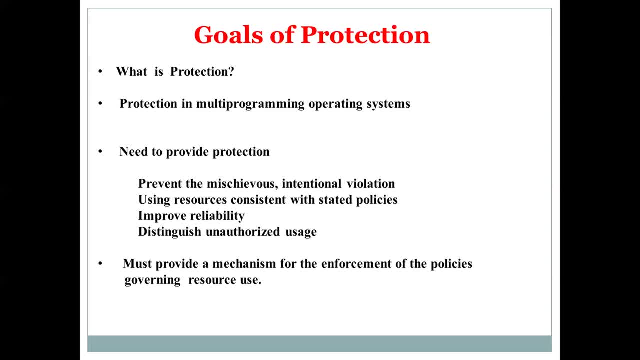 protection is a mechanism for controlling the access of programs or processes or users. call it whatever you want: it's a mechanism for controlling the access of programs or processes or users to the resources defined by a computer system. you are going to have different programs, you're going to have different resources. how these different? how we are going to control the access. 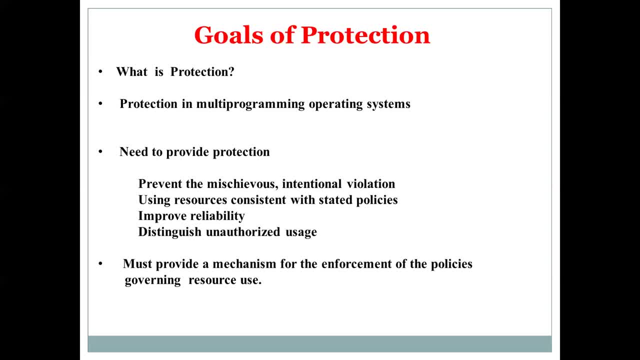 of these resources by the programs or processes. that is that mechanisms are called protection mechanisms. so protections mainly deals with access, controls of the resources, and not only that. protection mechanism must also specify what controls we are going to impose on the resources and how it is going to be imposed, what controls are going to be enforced and how the controls are going to. 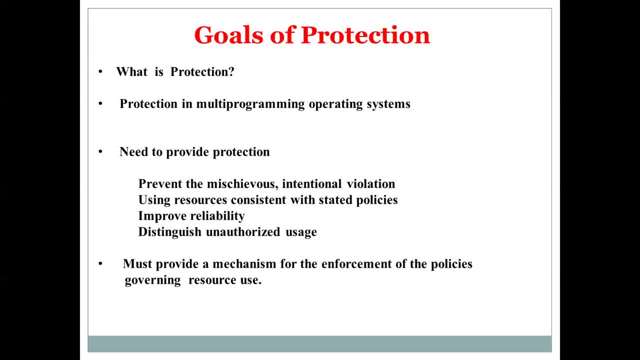 be enforced. so that is about the basic definition of protection. the next we'll move on to the goals of protection. so here i have listed out the different types of goals for protection. the first important need for an operating system to provide protection is: the first reason is to prevent intentional violation of an access restriction by a user. okay, you. 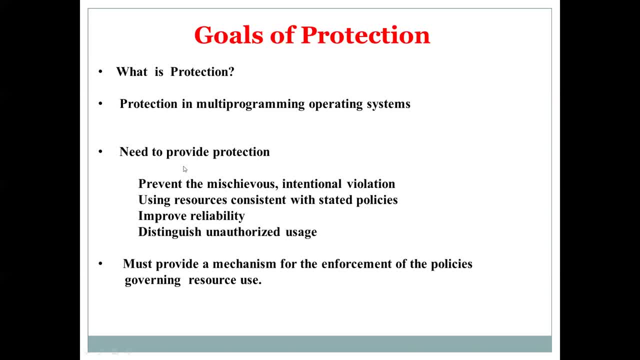 may have many malicious users trying to attack your system or trying to intrude into your system. So main goal of the operating system is to prevent the intentional violation of the access restrictions by a user. You have some access restriction. you have some restriction like a particular file cannot. 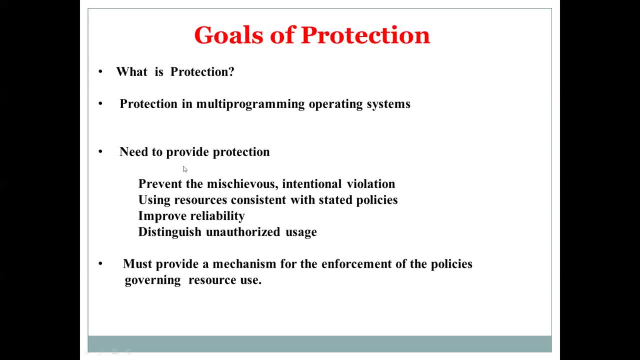 be accessed by a particular user. So if the user tries to intrude into that, violate into that. that should be avoided. That is my first goal. The second goal is: in many types of computer systems there may be many stated policies. 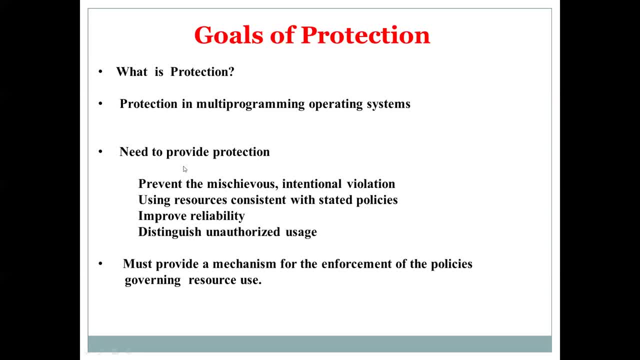 for resource usage. So the protection is used to ensure that every active program component in the system accesses the resources in consistence with the stated policies. For example, in many organizations you may have identity based resource policy, like, for example, based on the identity of the type of the user, he may be granted or reprimanded. 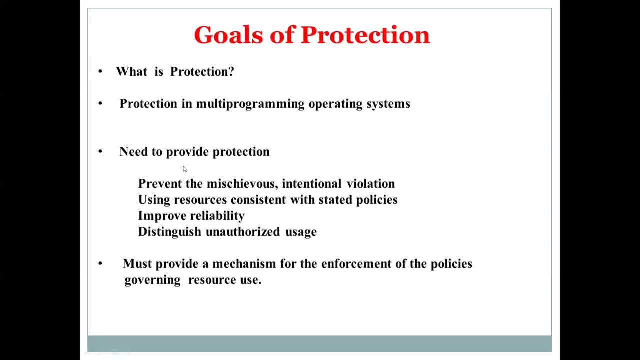 or denied access to a resource. In some organizations you may have resource based resource access policies. that is, for a particular user, who are all the resources? who are all the for a particular resource, who are all the users who are allowed to access the resource, or who are all the users who? 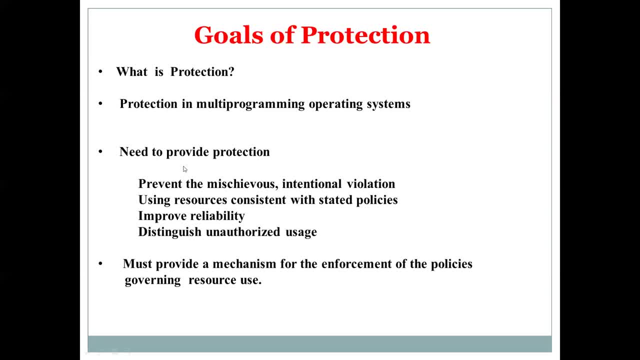 are not allowed to access. So that type of policy is called resource based access policy. So, whatever there may be some stated policies for accessing resources And then by protection we ensure that the resources, the all the active resources, are protected. All the system components in the system use the resources in consistence with the stated 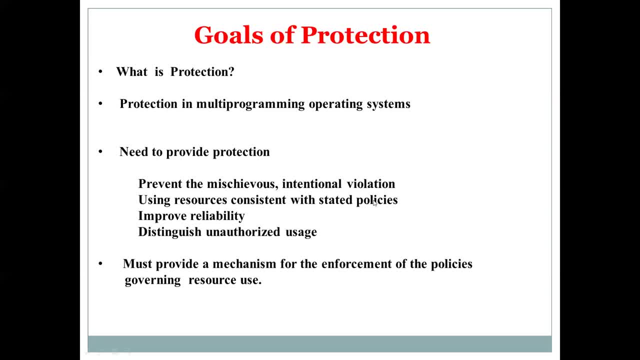 policies. So that is the second goal of protection. The third goal of protection is to improve reliability. So how protection can improve reliability is one example is it can be used to identify the latent errors at the interfaces between components of systems. That means when many subsystems are connected together, then there is a high possibility. 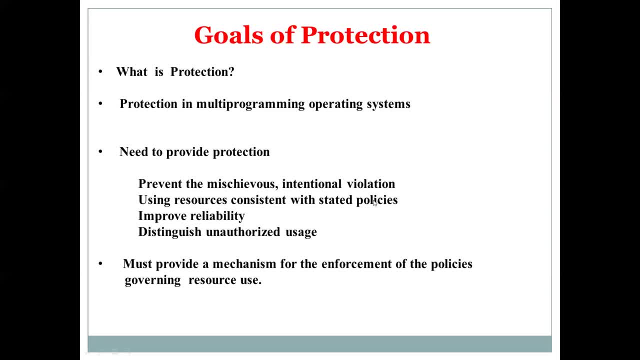 of some less apparent design design errors at the interfaces between those components of systems. Okay, you may have some. you may have some errors at the interfaces. Those are called interface latent errors and it's very difficult to identify those errors. So, if so, by using this protection mechanisms we can identify such latent errors and by 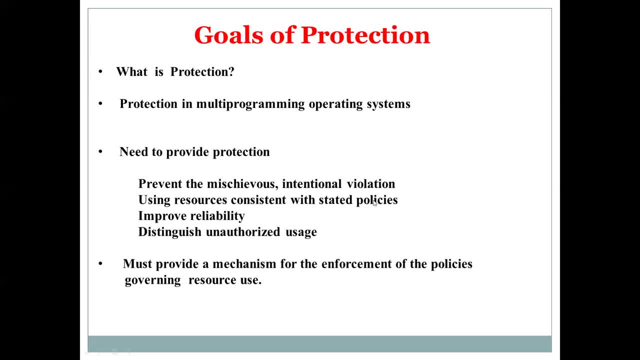 identifying that we can improve the reliability of the system. So by identifying that we can also do one more thing, We can also do one more thing, Okay. So we can prevent a healthy subsystem from being affected by a faulty subsystem. So that is the third goal of providing protection: improving reliability. 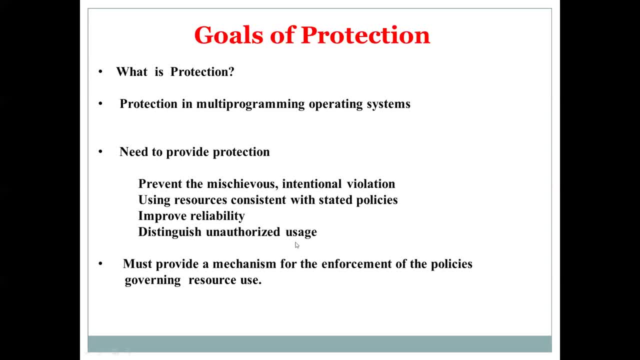 The fourth goal of providing protection is by using protection mechanisms. the system is able to distinguish between authorized usage and unauthorized usage. Okay, So, whatever may be the protection protection schemes which are used system should also provide a mechanism for enforcement, So enforcement of the policies governing the resource usage. 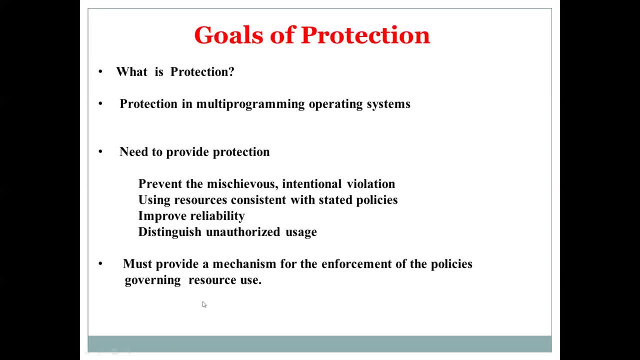 Now here you have to understand the difference between what is mechanism and what is policy. So policies actually specify what has to be done for protection and mechanism specify how it will be done. Yeah, So you can have some policies- resource access policies- in the organization. 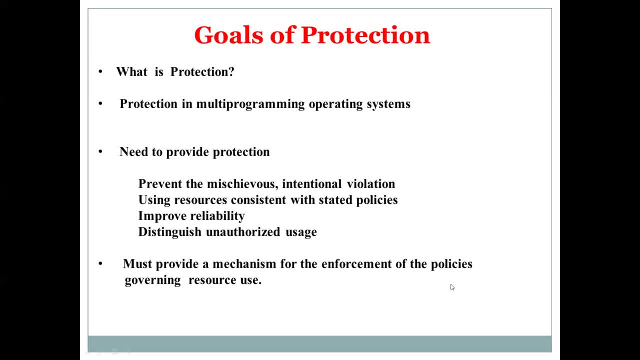 They are called policies. Policies will specify what has to be, policies will specify what has to be done, but then how it is going to be implemented is specified by using the mechanisms. so that is all the that is. so a role of protection is to. 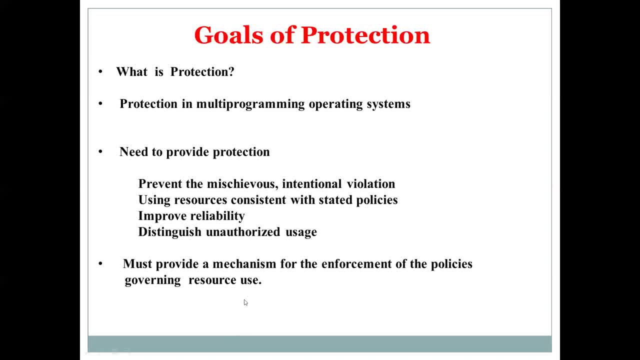 provide a mechanism for enforcement of the policies governing the resource usage of the organization, so that mechanisms can be implemented at different stages. it can it may be implemented during system design stage, or it can be implemented during system management stage, or we can leave it to users so that they can enforce protection when they make use of their. every individual user can. 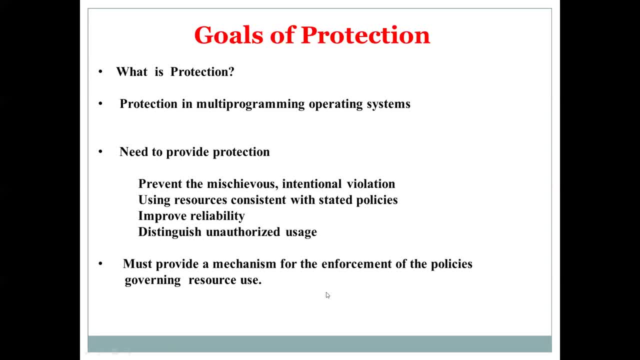 enforce protection for their own files or for their own programs, so we can leave it to the users also. so your protection mechanisms must have some mechanism for enforcing the policies, but then it can be implemented at any stage. that is up to the operating system. but then some mechanism. 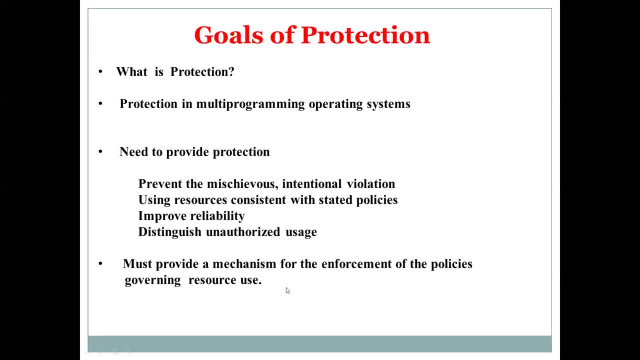 should be there for enforcement of the protection policies. so these are all the different goals of protection. so, to conclude, we saw what is the meaning of protection. so protection is nothing but a mechanism for controlling the access of programs or processes or resources by the sorry. protection refers to mechanism for controlling the access of resources by the 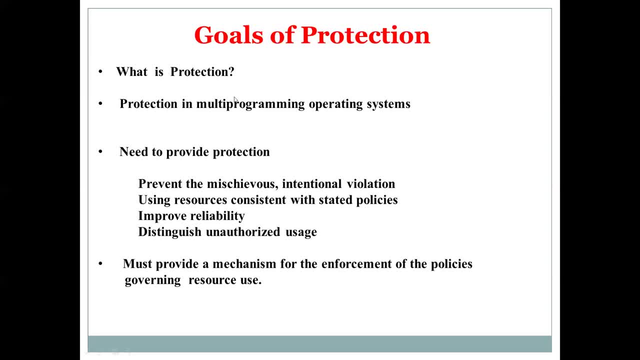 programs or the processes or the users of a computer system, and we saw the different goals for providing protection. one goal for providing protection is to prevent the intentional violation of any access restriction by a user, and the second goal of providing protection is to check out and to ensure that all the resources are accessed by the any any active component present. 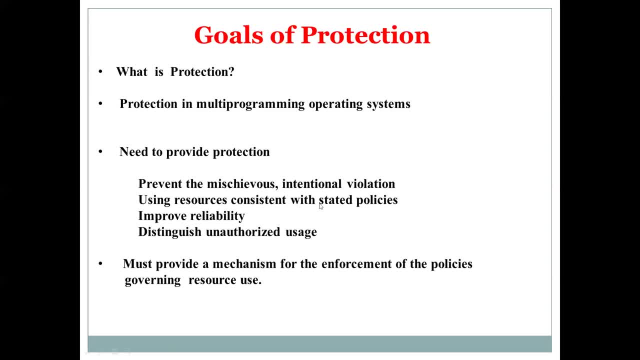 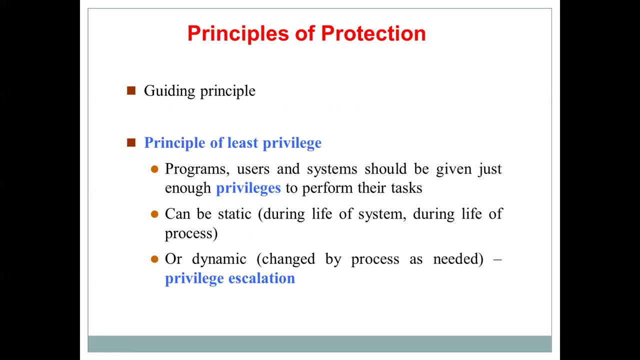 in the system. any active program component uses the resources in consistence with the stated policy. and the third one is to improve the reliability by identifying the interface errors. and the fourth goal of protection is to distinguish between authorized usage and unauthorized use. and finally, to remember all those notifications. so another little thing to mention is ИЗ sl. 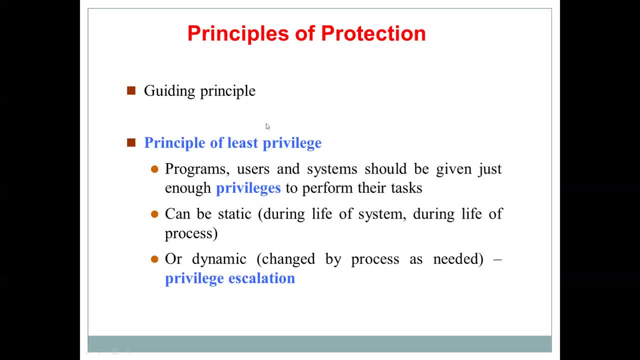 project design so that the system becomes consistent and easy to understand. okay, so let's say you are designing an operating system, a new operating system. your guiding principle will tell you guidelines for implementing that operating system so that your system is consistent and easy to understand. okay, without it is like guidelines, without guidelines it is. uh, it will. 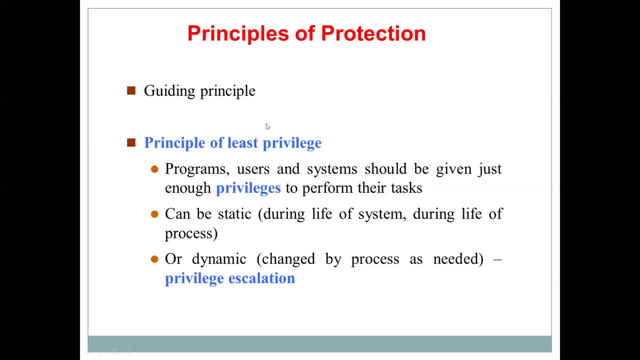 be very confusing for the designer to know where to start or where to complete and or what, what guidelines to follow. okay, so a guiding principle is nothing but a principle which you can use throughout the design of a project so that your resultant project, or the system becomes. 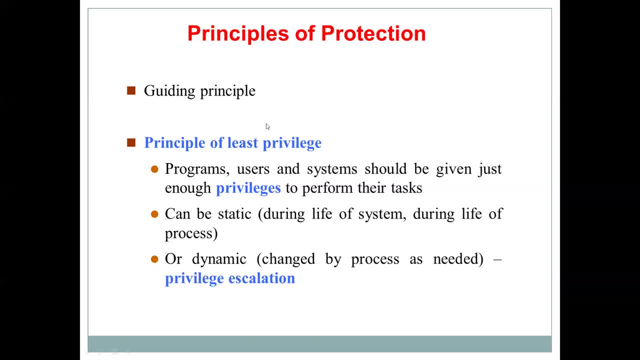 consistent or easy to understand. that is called guiding principle. now, what is the guiding principle used by operating systems for protection? that is called principles of protection. by principles of protection i mean what guiding principle is used by the operating system to enforce protection? okay, the guiding principle used by the os to enforce protection is called as principle of. 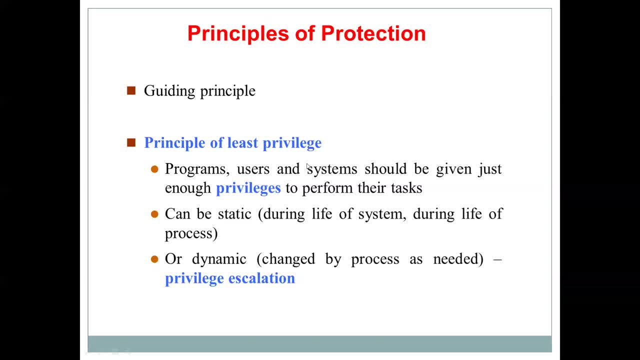 least privilege. principle of least privilege is the guiding principle used by the os to enforce protection. now, what is the meaning of this principle of least privileges? it says that to all the programs or the users or the systems, just to give just enough privileges to perform their tasks, whatever may be the number of programs or users or systems, just provide them with the. 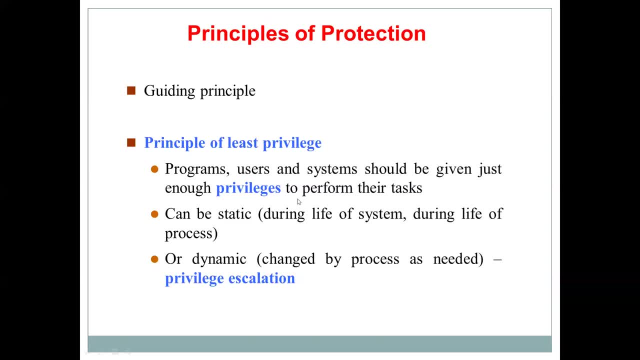 just enough privileges to perform their tasks. now, what do we mean by- just to try to remember this term- just enough privileges? principle of least privilege says that just give, just provide, just enough privileges for the programs or users to perform their tasks. what do i mean by that? an 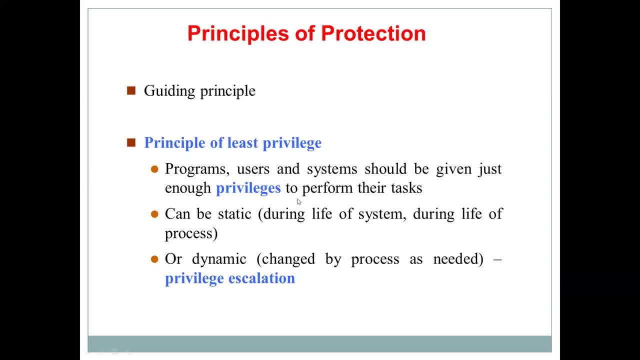 analogy is: let's say, i have my house keys and i have to give it to some third person and i don't have any other option other than giving it to the third person. so here, if i decide to give, if i give public area of the house, then in case if the keys are lost or if it is compromised or if it is stolen, 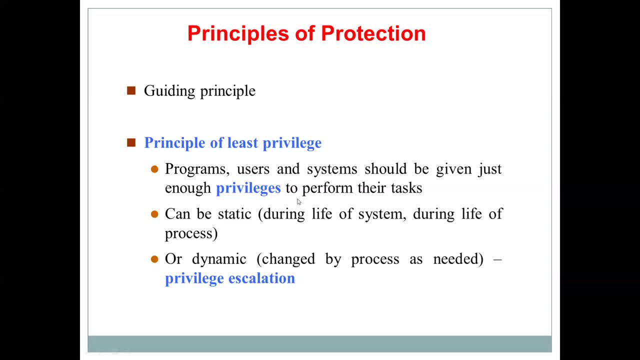 or if it is misused by the third person, but then the damage is going to be less okay. on the other hand, let's say i give all the keys of my house, both the public area keys as well as the private area keys- then then what will happen in case if the key is stolen? i'm going to get maximum damage in case if the key 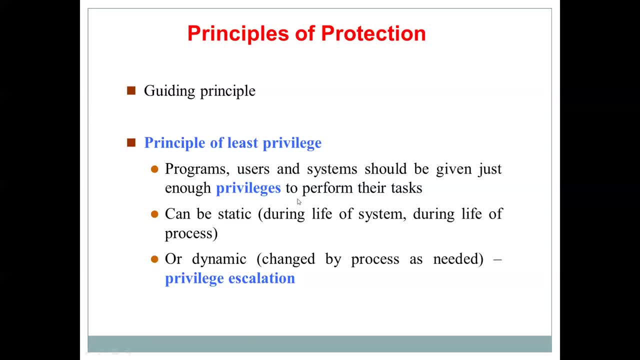 is stolen or compromised or misused by that third person, i'm going to get maximum damage. so what i will do is if i give only the keys of the public area of my house so that the damage in case of fault is minimum, then that is called principle of least privilege, principle of least privilege. 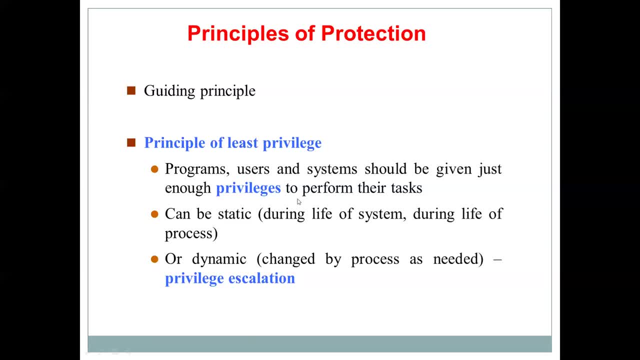 that is the principle of least privilege. it says that give only the, give only that many, that much amount of privileges that is enough for the program or the user to perform, to complete his task. don't give too much privilege. um, if your home damage is minimum, then it is the principle of least privilege. 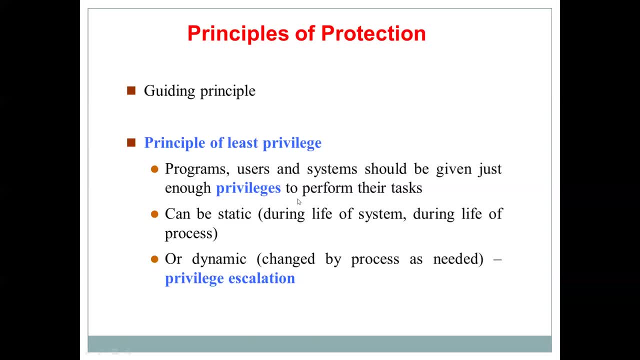 so that if there is any fault, then the system will have to incur maximum damage. That is the principle of least privilege. Now, when can this least privilege can be established? It can be established in two ways. One is it can be static or it can be dynamic. 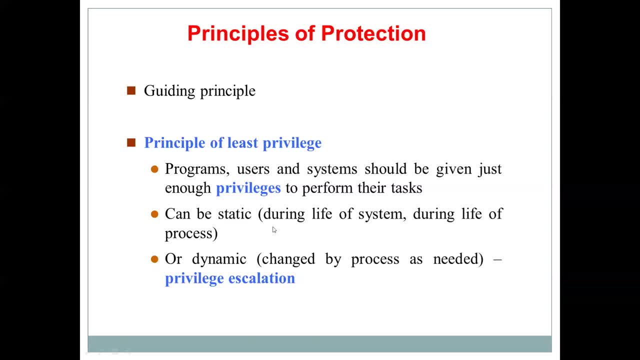 By static means that for entire system, lifetime or for the entire process, lifetime. if I establish some principles to be followed, that is called static privilege. The other type of privilege is dynamic privilege, That is, the privileges are not going to be same from time to time. 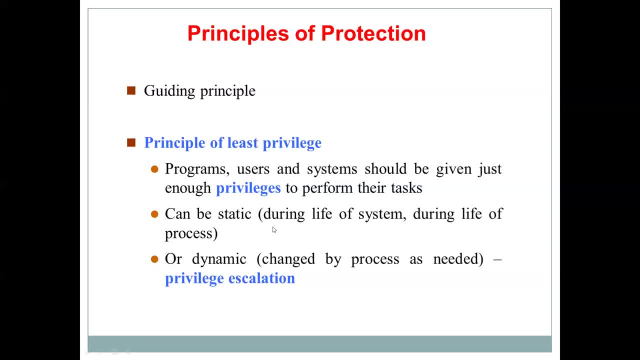 Depending on the need of the process, the process is going to change its privileges. That type of assigning privileges is called dynamic privilege. One example is privilege escalation, where if some process has lower privileges, it may be assigned some higher privileges depending on its need. 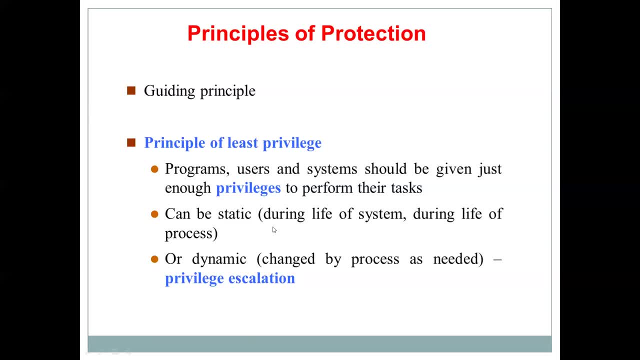 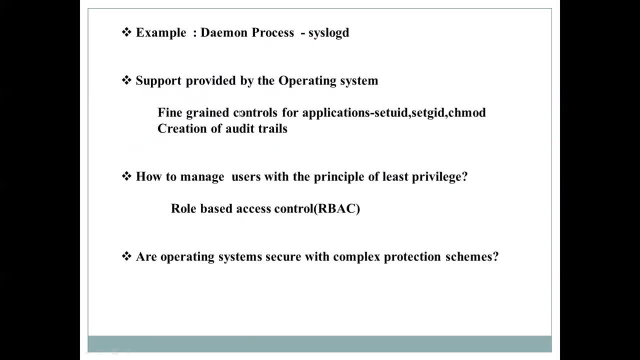 So let's see how operating system will enforce this task of the principle of least privileges. What are the requirements for the operating system to enforce this? So, as an example, consider a daemon process. We all know that daemon process. there are many different examples of daemon process. 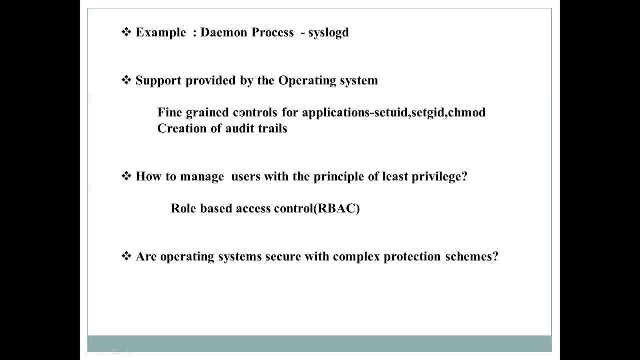 You may have daemon. we all know that daemon processes run in the background without any user interaction. So we may have a daemon process to just monitor the network activity or to take log of the suspicious network communication. Or, for example, we have a daemon process called as syslogd. 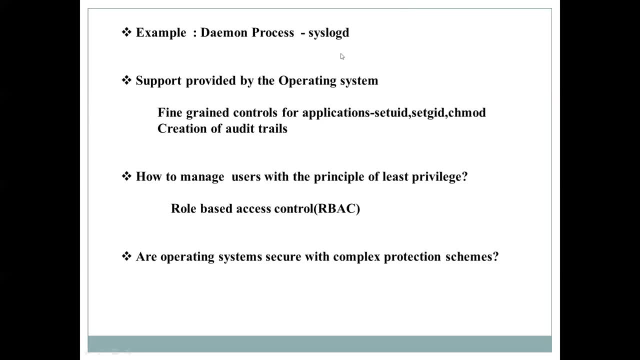 So this syslogd in Unix system is used to implement. So this syslogd in Unix system is used to implement the system login logging facility. So in case, let's assume that there is some fault in the daemon process, that there may be a fault like a buffer overflow or something like that- 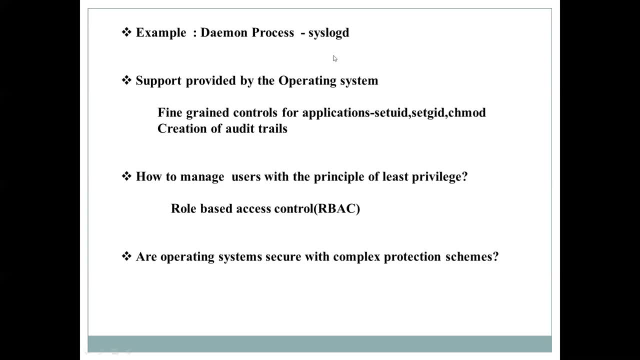 So, in case, if there is such a fault, it may cause the daemon process to fail. In case if the daemon process fails, I have to ensure that any remote user should not be able to gain full access to my system Or, because of this failure of the daemon process, any remote user should not get maximum privileges because of this failure. 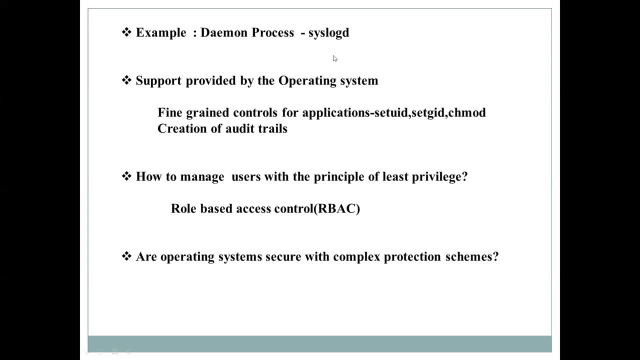 Or because of this failure of the daemon process. any remote user should not get maximum privileges because of this failure. Okay, So that has to be ensured by the system, And that is one example of using principle of least privilege to ensure that the damage is less. 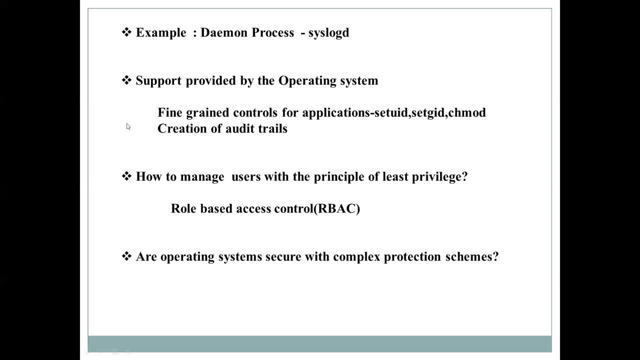 So for this, what are all the support which is provided by the operating system is: Operating system provides many system calls for applications, So it allows it provides for many system calls and data structures for the applications to have fine grained controls. So what is the meaning of fine grained control is: 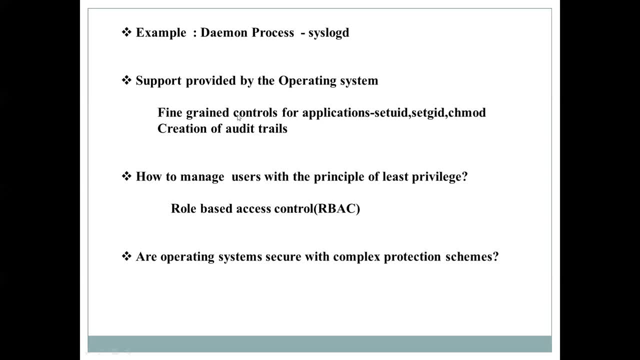 For example, let's say I have one analogy is: let's say I have the volume control knob of my speaker. So if I am able to set my volume control knob to exactly the volume- I want- exact volume, I want not too low volume or not too high volume- then I would say that my speaker is 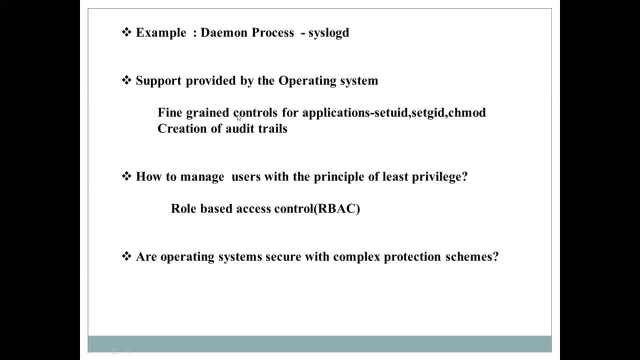 having fine grained control. Okay, If I'm not able to set the volume to the exact desired level I want, then I will say that my application is not having fine grained control. So some examples of some system calls: it is provided by operating system for this. 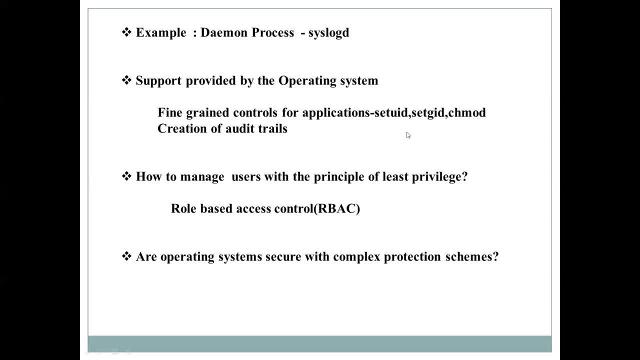 So how operating system provides. this is operating system provides- system calls for the users to enable privileges or to disable privileges. We would have learned a lot about these type of system calls right. One such example is our CHMOD system call. So this is used to change the file access permissions. 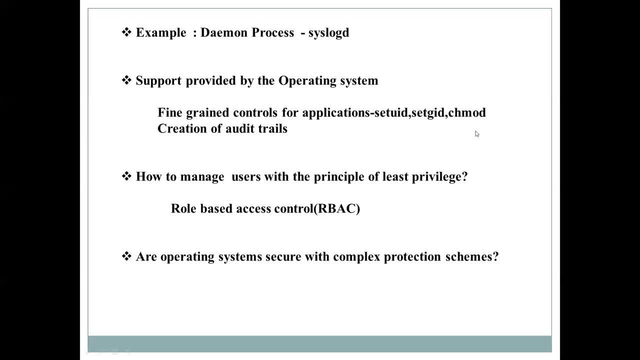 Okay, So by that the applications can be given privileges. So if the application is enabled we can disable the privileges. Similarly, another example is the set UID and the set GID system calls in units. So with this system calls any program which is starting a root can run with reduced system. 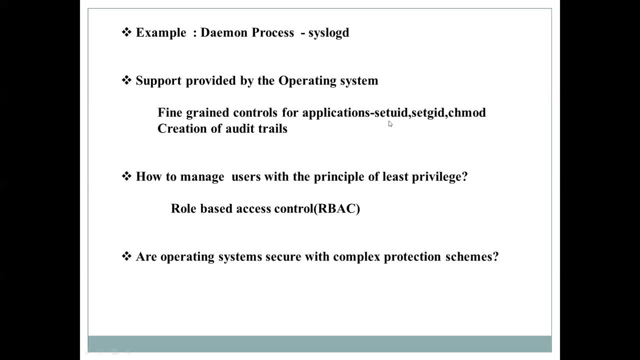 privileges. We can give some privileges for a program which is going to start as a root user but then, but still, it can continue with reduced privileges And with that we can reduce the damage, amount of damage which can happen if there is a. 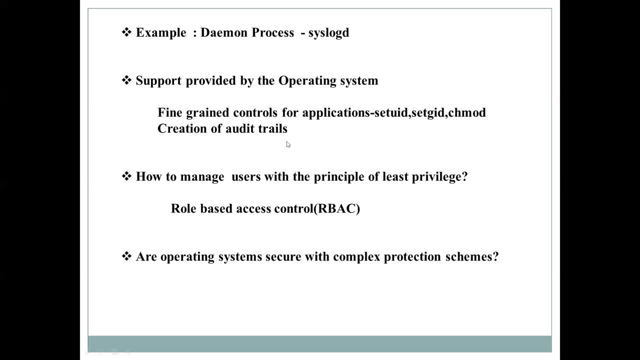 fault, Okay, Okay. Another way in which the operating system it can also run with reduced system privileges- Okay, provides support for this principle of least privileges- is by using, by creating audit trials. now, what is the meaning of this audit trial? is it ensures that 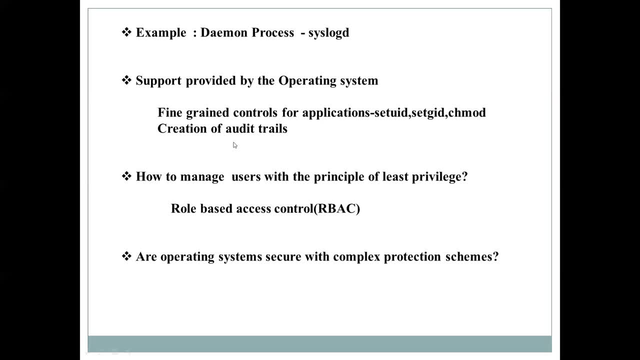 audit trial is nothing, but it keeps track of all the changes which has been made for database or to a file. now here, by maintaining audit trials for all privileged function access, the OS maintains audit trials for all type of privileged functions access. so what is the way is going to gain by creating: 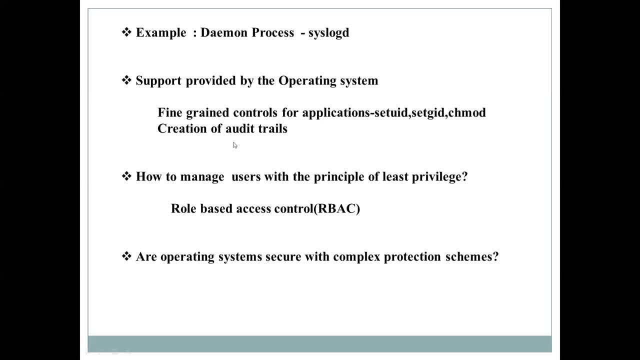 this audit trials whenever. so it allows the programmer or a system administrator to trace all the protection activities and security activities on the system and whenever there is any violation it can be easily detected. so support by the operating system for ensuring the principle of least privilege is done by. 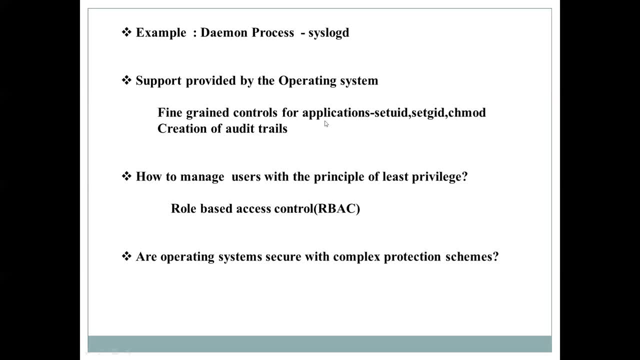 using two ways. one is by using appropriate system calls provided for applications and the other is by using the system calls provided for applications. example, is your phmod set UID or GID system calls? and second is operating system maintains audit trials with which any system administrator can can keep. 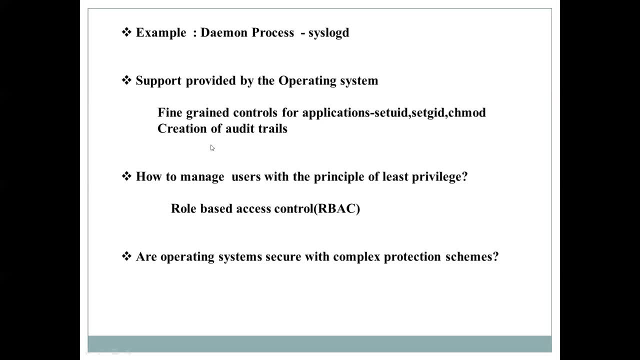 track of all the security activities of the system. and the next thing is: similarly, operating system also maintains, manages users, with this principle of least privilege. how it manages users is by creating a separate account for each type of user and providing role-based access control. what is the meaning of role-based access? 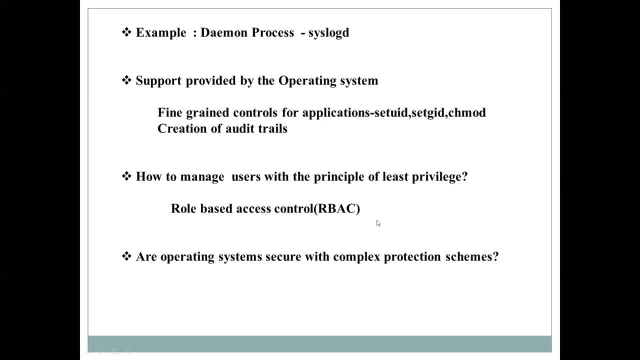 control. depending on the role of the user, he will be given access control and by that the OS ensures the principle of least privilege. one example is: let's say I have a system operator whose job is to mount the backup files onto the system. now he will be given only the commands. he will be having restricted access. he will be 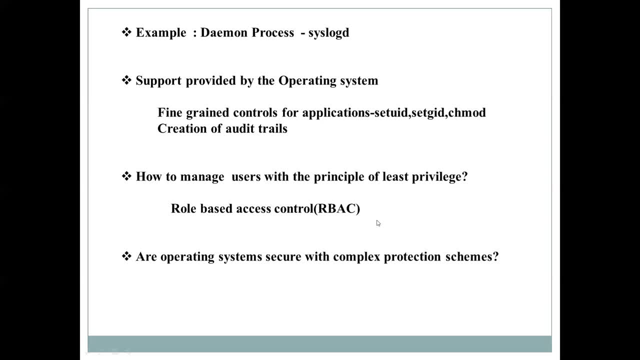 given given access only to those commands, voices and to those files which he requires for the mounting operation. the operator- system operator- will be given access only to those commands and those files which he requires for the system access. he doesn't need access to any other comments because this job is only to do the mounting operation after. 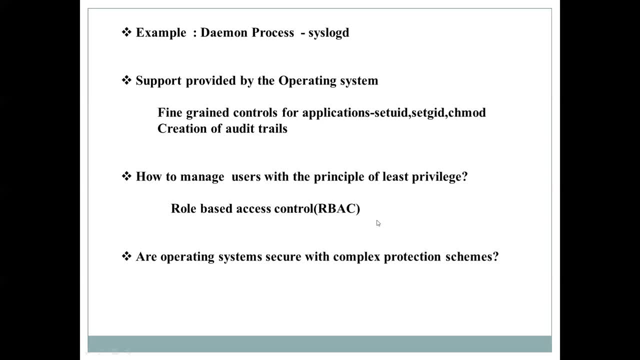 corresponding backwards. so that is called us role-based access control. so by creating separate accounts for separate types of users, who is also ensures the principle of least privilege. and finally, to creating separate accounts for different kinds of users, to un-allocate each inside to a specific module for each user too. 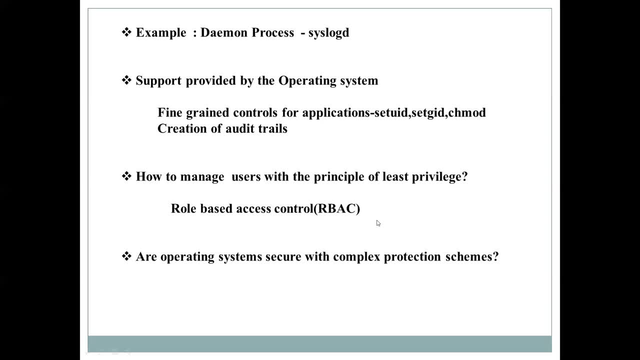 the principal of Aifies to privilege. and finally, the principle of least privilege's is evangelize friendship, because to create a recommender and to create a dreaming member, goal To um với the principal of least privilege to a given user as an employee, the. And finally, to conclude, if we have to check whether operating systems are secure by all these different types of complex protection schemes, the answer is no. 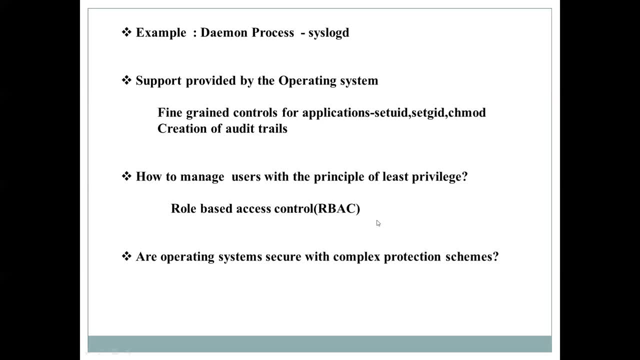 One example is your Windows operating system. Windows operating system has a lot of complex security protection mechanisms in itself, just like this. But then we know that Windows has a lot of security loopholes. Maybe it is because of the fact that it is protecting the wrong aspects of the operating system, or since because the code which it has to protect is vast- it has many lines of code- and so it is not able to provide the complete protection.